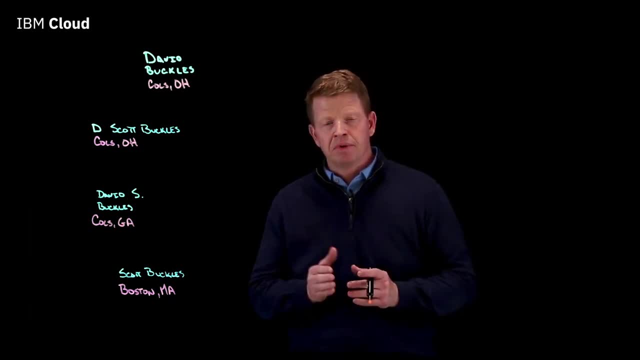 It's been a long flight, Got a great greeting from the bellman as he opened the door And as I passed through the lobby. I have trepidation to know whether or not all the requests that I've made as part of my reservation. 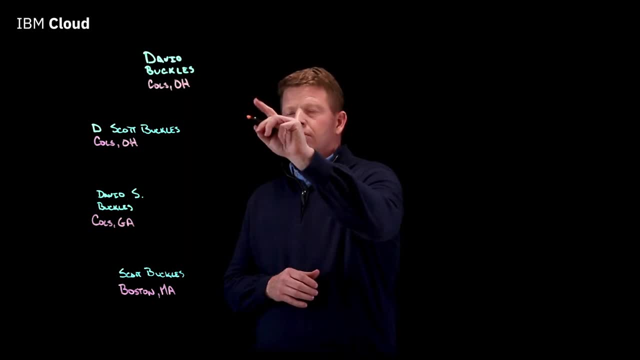 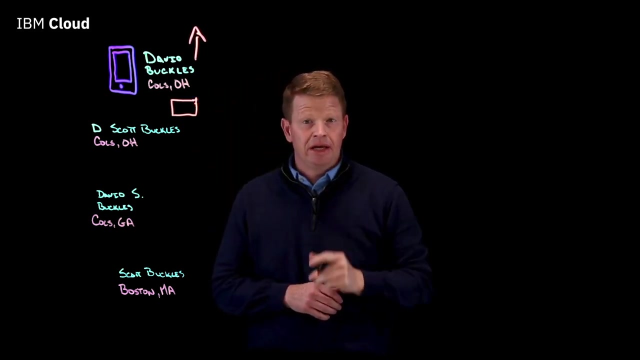 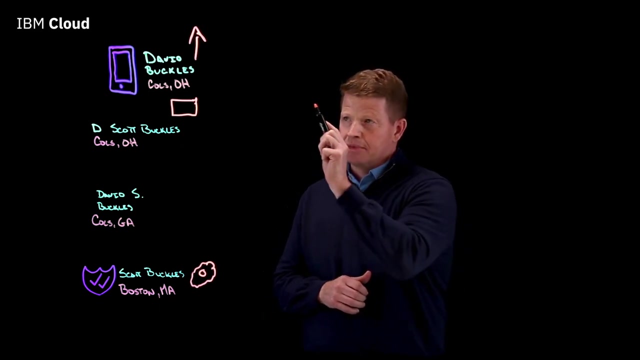 will be made. When I booked it on the app, I requested a high floor. Traditionally, I've always asked for fluffy pillows And then, as a super-duper titanium member, I always want my free breakfast. In order to do that, we have to be able to determine that I am the same David Buckles. 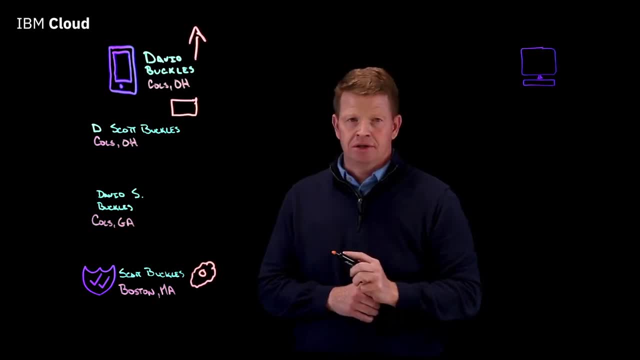 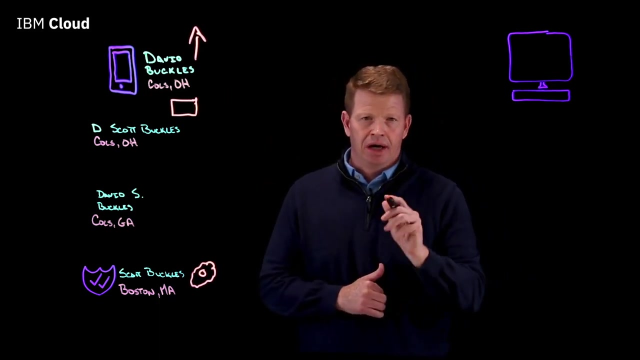 across each of these different applications and that when the front desk checks me in, they've recognized that and incorporated all of my different requests. Let's take a deeper look In the mobile app. I'm David Buckles from Columbus, Ohio. 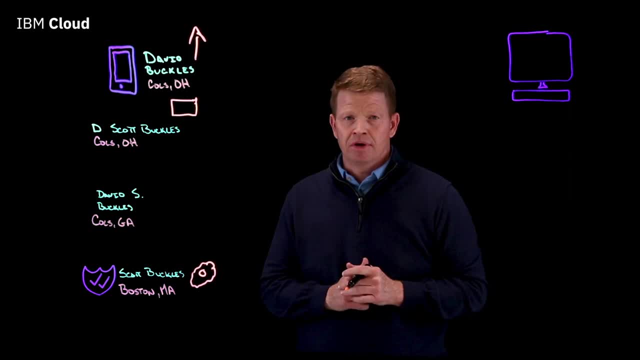 because it's time-consuming. I'm a student at the University of Michigan and I'm a student at the University of Michigan, and I'm a student at the University of Michigan and I'm the head of the Library of Michigan. That's tied to my credit card and that's how the reservation was booked. 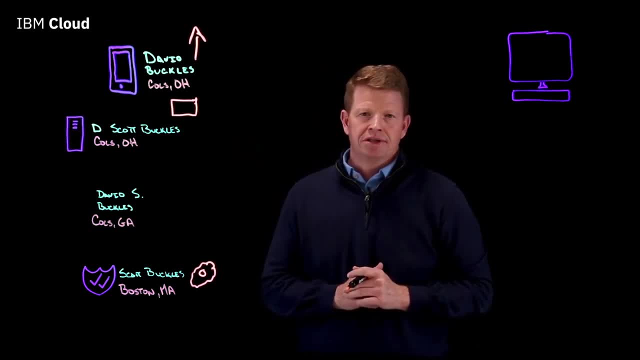 In the past in the legacy reservation system I've booked rooms as D Scott Buckles, And that is where my fluffy pillow request has always come in. I've also had somebody with the name David S Buckles from Columbus, Georgia, call in. 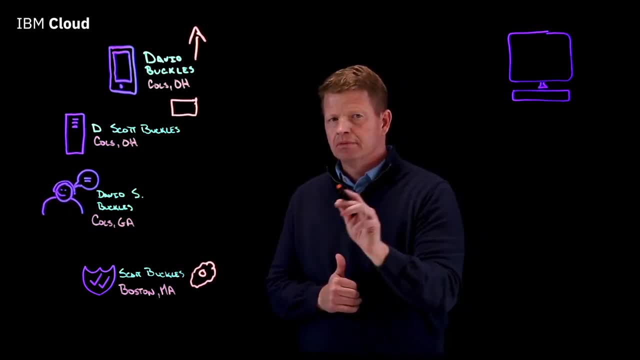 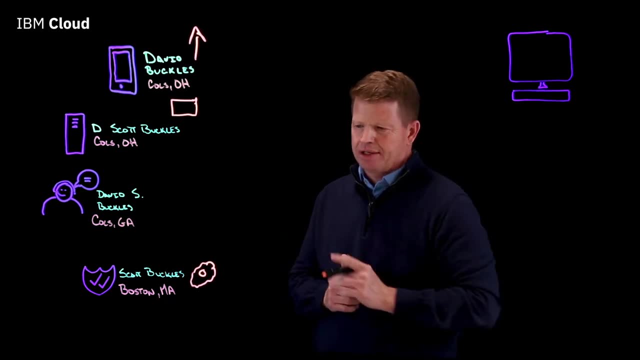 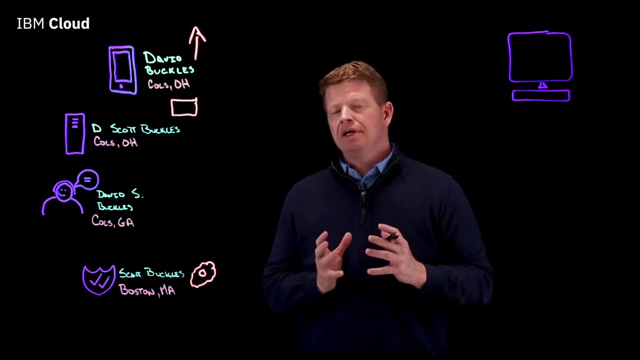 Is that me or is that a different David Buckles? Stay tuned. And finally, in the loyalty application, when I first signed up, I lived in Boston, Massachusetts, and I entered under just my common name of Scott Buckles. MDM solutions. at their core are algorithms. 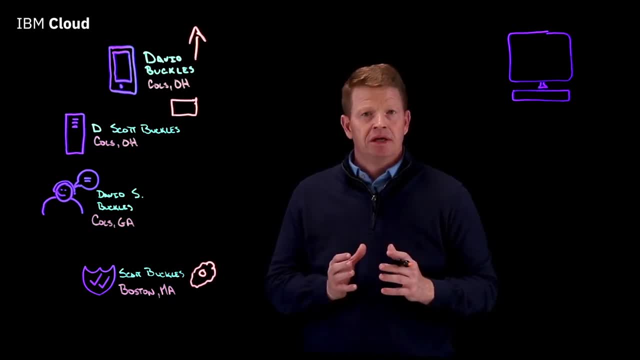 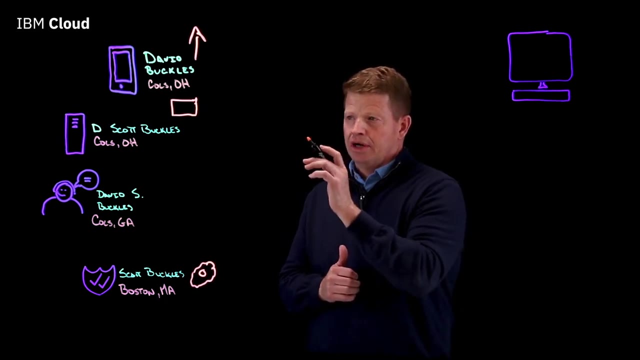 They take different parameters and different rules to determine if a person is the same person with different data entry points, such as David Buckles D, Scott, David S or Scott Buckles. A good MDM solution will be able to determine whether I am the same person across all four of these or maybe it's just three of the four.